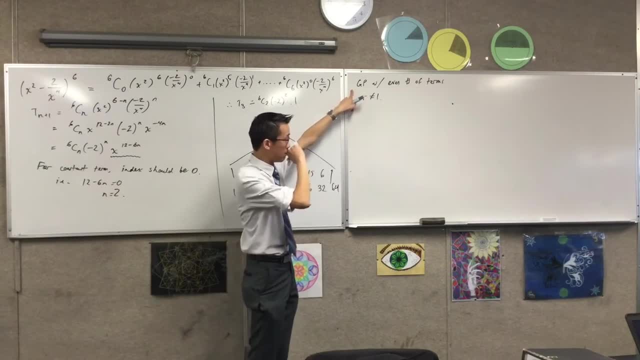 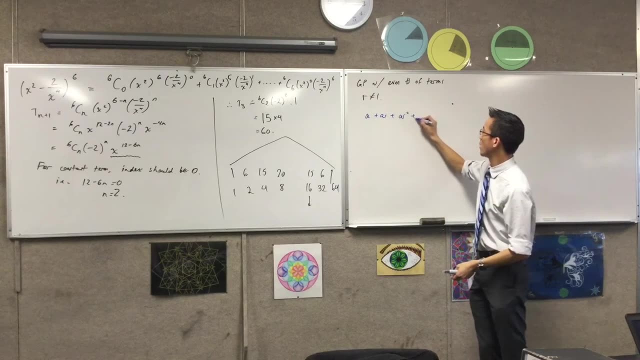 So here's where I'm going to start. There's a GP. It has an even number of terms. Every GP is in this form: right: A plus AR plus AR, squared. I'm going to do another term just for the sake of it. 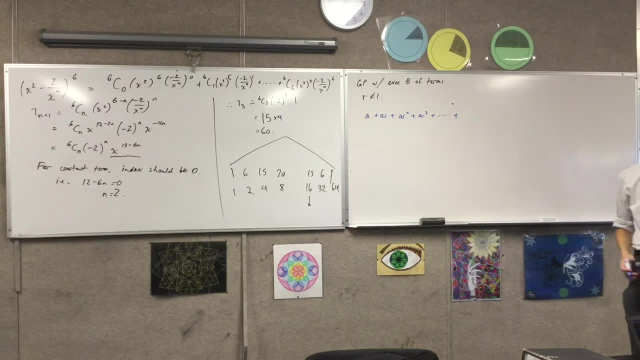 What will my last term be? My last term, the nth term would be AR to the M minus 1.. Now, for reasons that will become clear in a second, and you'll probably be asking, like I know, to write this, and the answer is: I didn't. 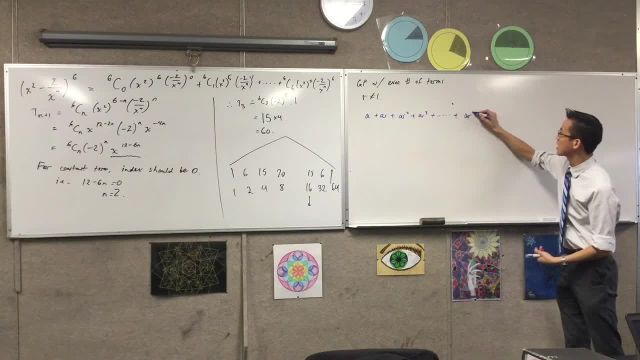 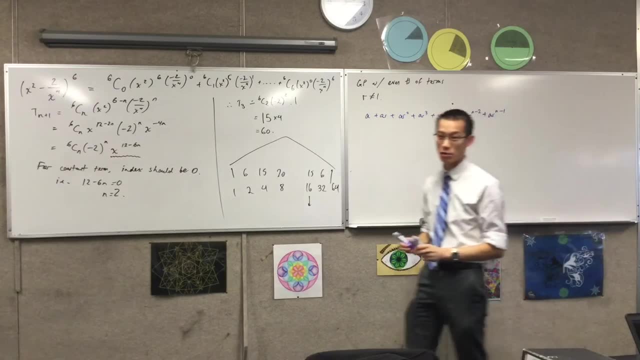 but I've worked out after the next couple of lines that I need it. I'm going to put the second last term in as well, which is 1 and less, and then here comes the last one. Does that make sense? So there's my whole series. 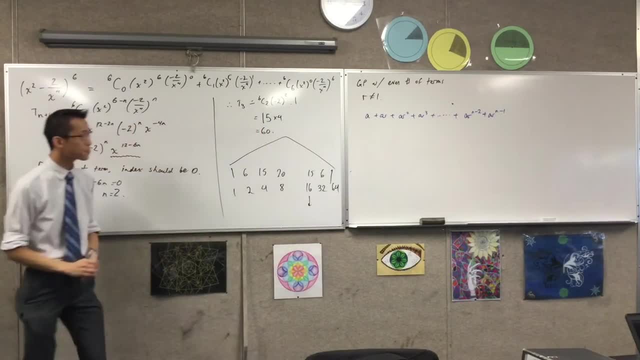 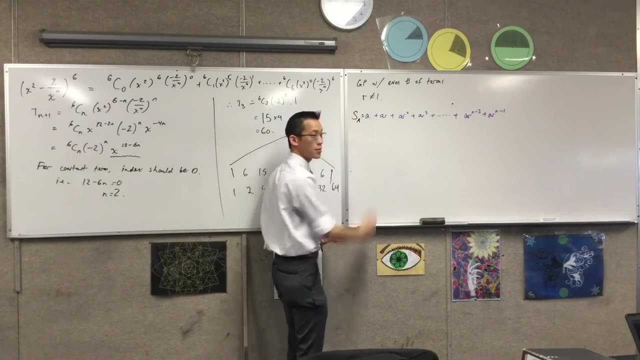 This could be any GP, right? I don't know anything special about this yet. That's the sum of the whole series. I'm going to call this sum of A for all terms. Now I want the terms in the odd places. That's the first, third, fifth, seventh. 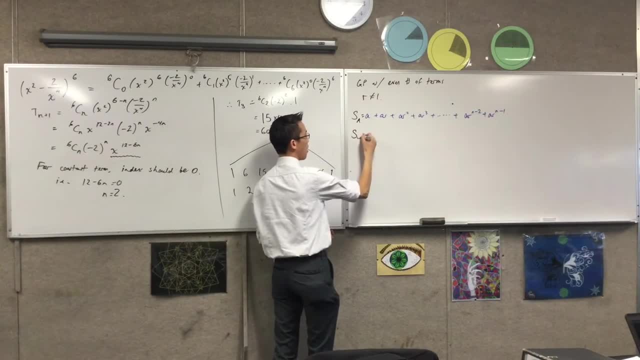 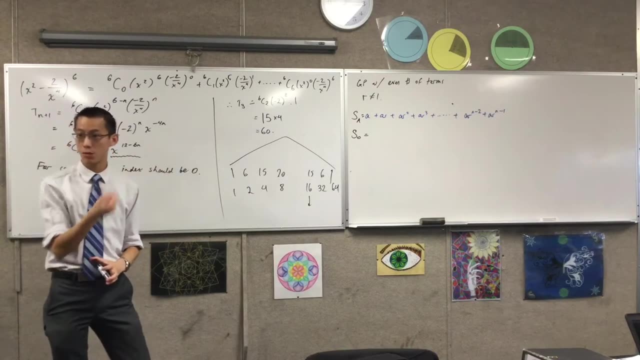 et cetera, all those places. So I'm going to call that the sum of the odd terms. Now you can see, and this is why I've written a few extra terms, I can pull out those odd terms quite easily, right? 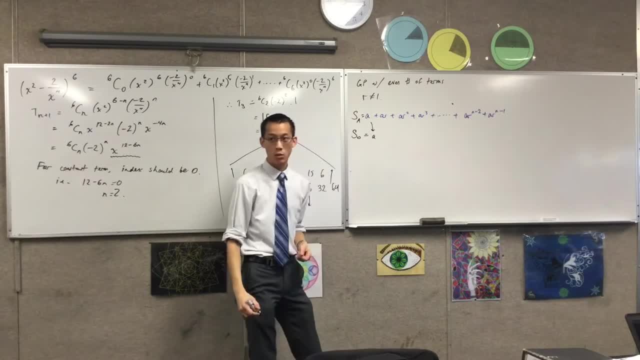 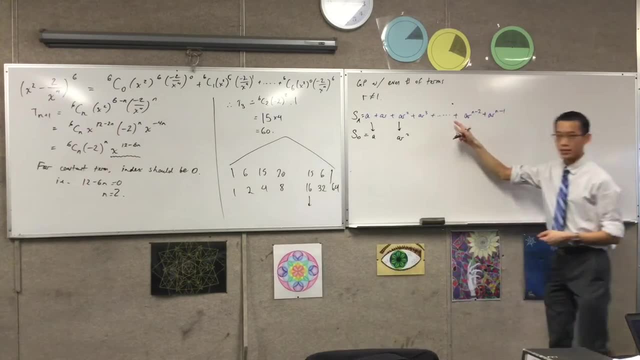 So, for example, here's the first one. That's pretty easy. What's the next term? I'm interested in this series: AR squared Now. my next one would be AR to the 4.. I'm going to leave that one. What's going to happen here? 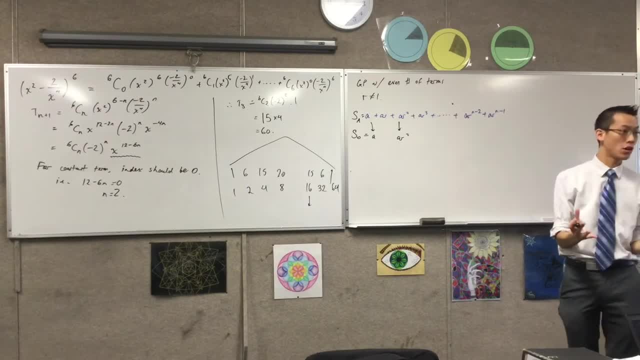 Which of these terms is the one that I want? Okay, This one has to be odd. Which one? Now, here's the thing. If I look back to the question, the whole GP, this thing has an even number of terms. 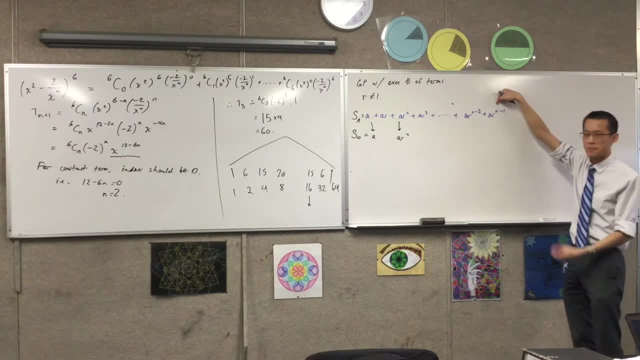 So, whatever that is, it's an even term. right, It might be the 20th term or the 40th or the 100th, but it's going to be even. That means this one has to be odd. Does that make sense? 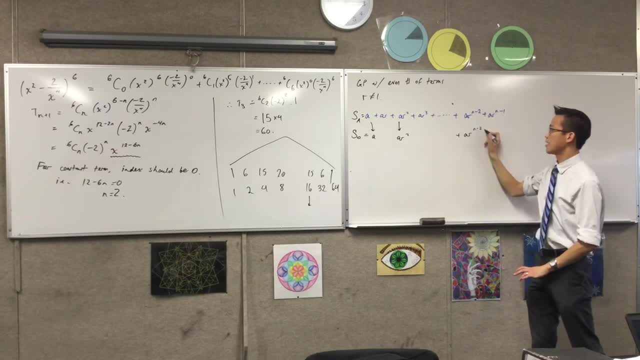 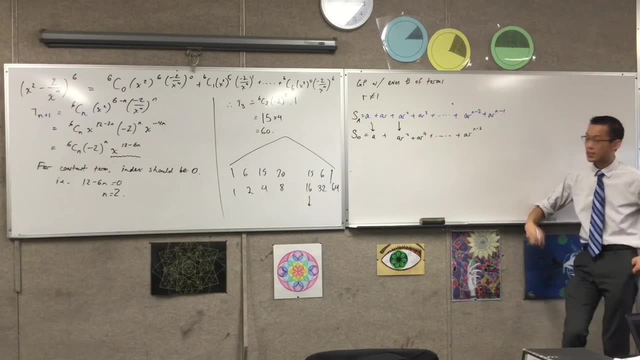 So the last term will be this guy. Okay, So, plus, I should actually put AR4 here, so I have a whole pattern. So this is what I've got. Okay, This is the sum of the odd terms. Okay, And here's what's really about this, right? 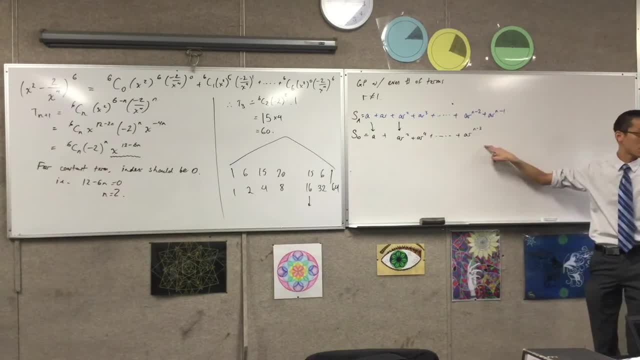 The question simply tells me that this is 5 times bigger than this. Whoops, There we go. So, in order to unpack this, I'm just going to say: well, hold on. the first term is any GP. It's any GP at all. 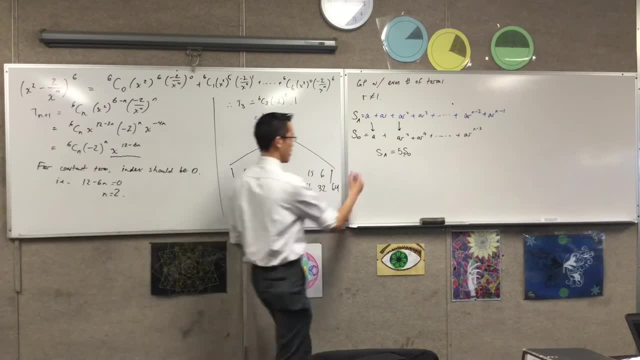 And I know what the sum of a GP is. It is A times what. Now I can say this forwards or backwards, It doesn't really matter right, But if I've got that on the numerator, then on the denominator I have. 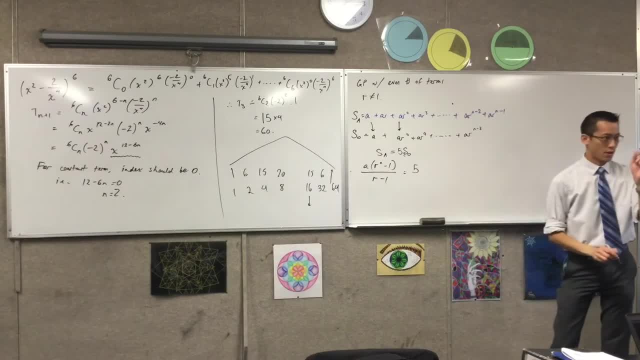 Okay, Now that's equal to 5 times Okay. Here comes the thinking: right? Well, it's the second piece of thinking. The first piece of thinking was recognising. that's the last term. The second piece of thinking is: what are all the pieces in this series? 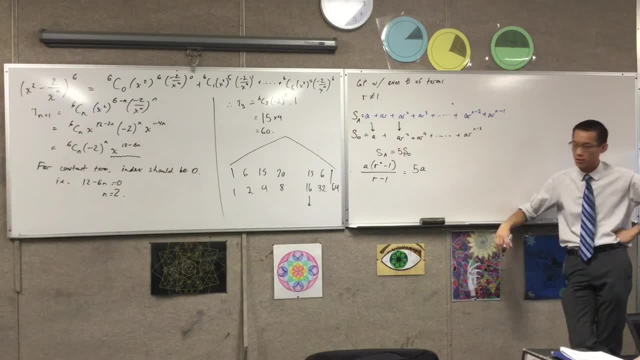 Well and easily enough. for me, the first term is still A. Okay, Then in here. I need to think about the ratio. I'll have a look. Yeah, you can see. every time I'm going by an R squared because I'm skipping terms. 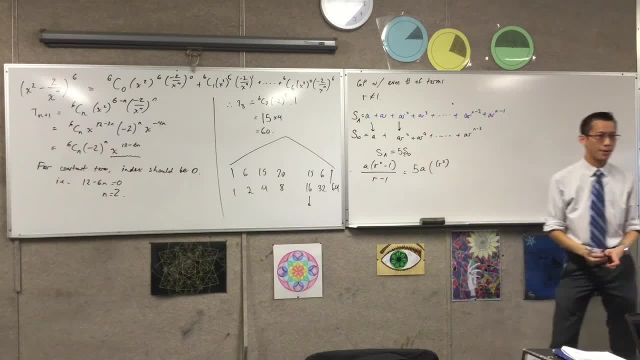 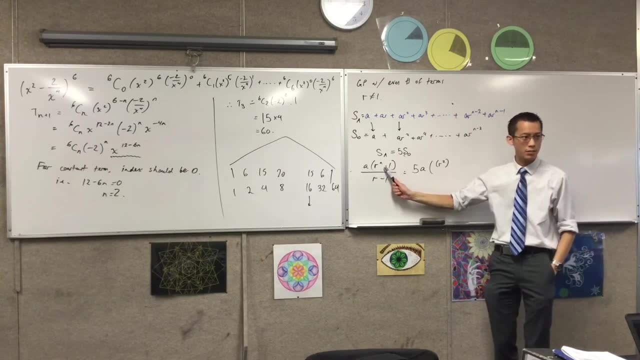 Does that make sense, Right? So in here, instead of R I write R, squared. Okay, Now pause for a second. If you see this immediately, don't shout it out. Let the rest of us think it through. How many terms will be in this series? 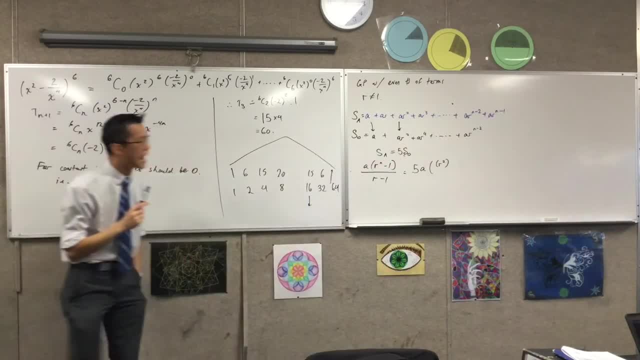 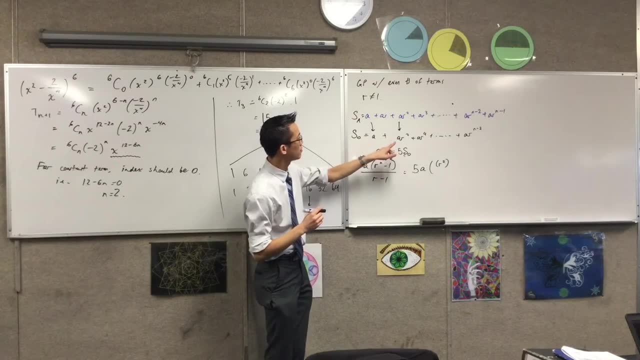 Stop and think about it for a second. Okay, Have a look at the way I've written it. Have a look at the way I've written it. Okay, Can you see, Am I even? Yeah, that's enough, That's enough. 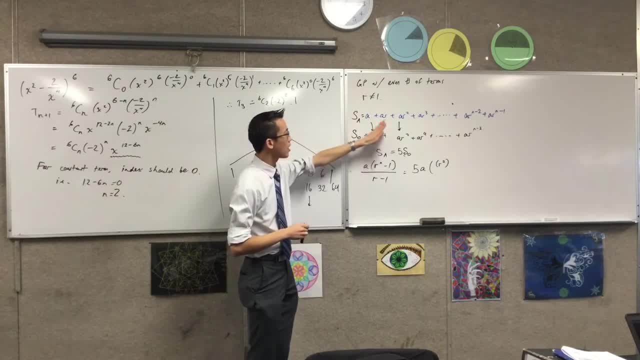 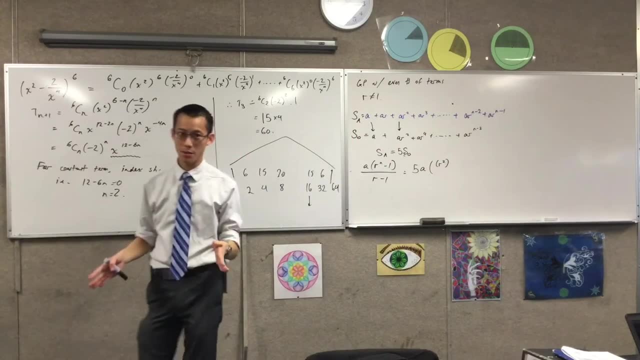 Can you see that when I form this series right, Every time I was missing a term, Missing a term, Missing a term? Do you see that, Because there is an even number of terms, every odd term is matched up with an even term? 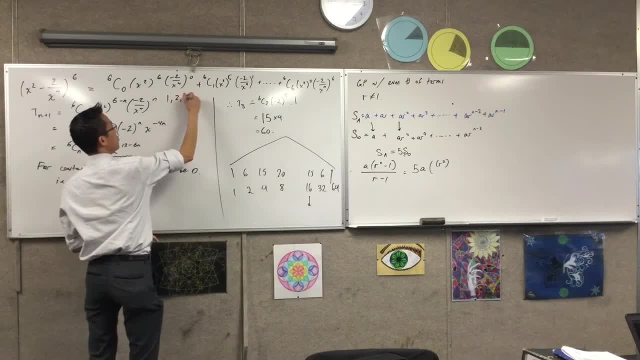 Right, If there was an odd number of terms, then I wouldn't know that. If there was like one, two, three, four, five, right, When I get these odd ones out, they don't all match up, Do you see that? 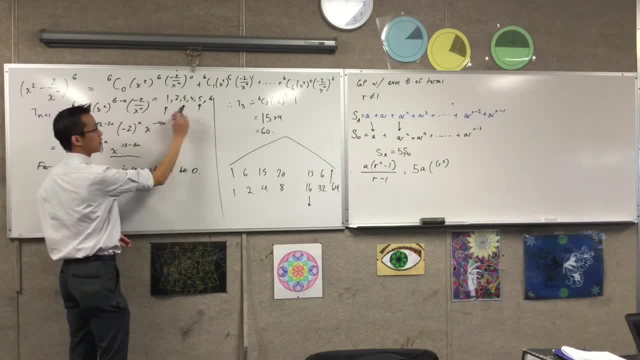 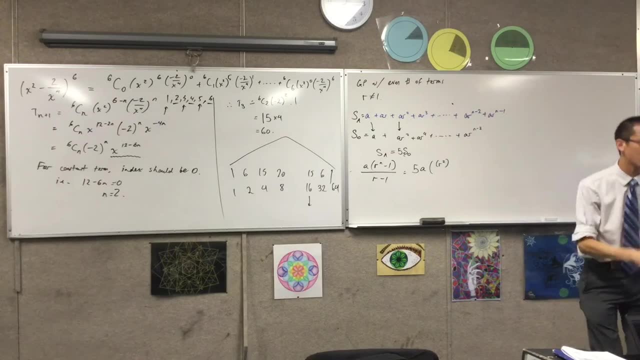 If there is an even number of terms, every odd term matches up with an even one. Do you agree with that? So that means, because there's an even number of terms, there must be exactly half the number of terms as there were in my first one. 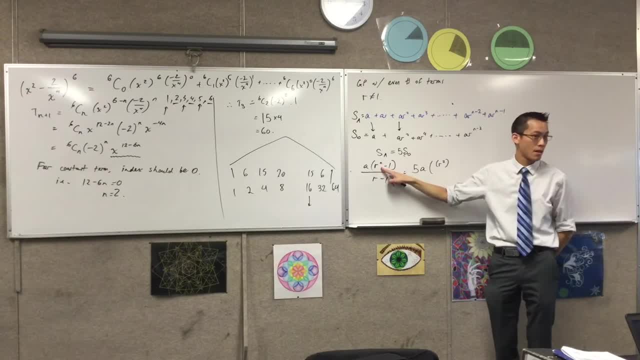 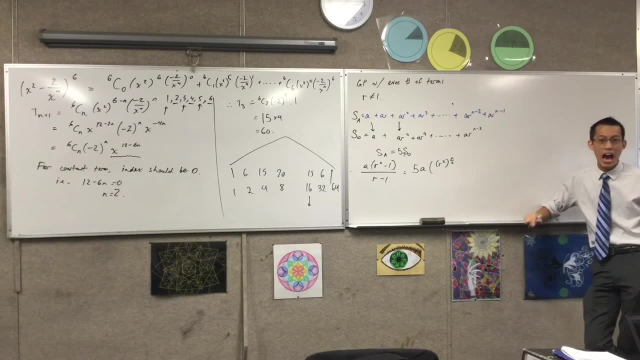 Okay. So if there were n terms last time, there's going to be n on two, n minus one, Right, Isn't there? n minus one on two? Actually, no, How many terms are in this series? All of those n? because it's three. 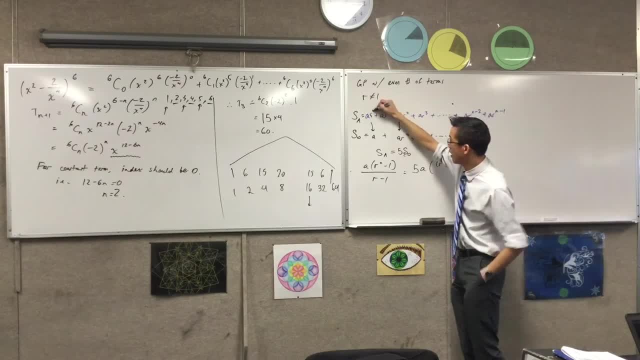 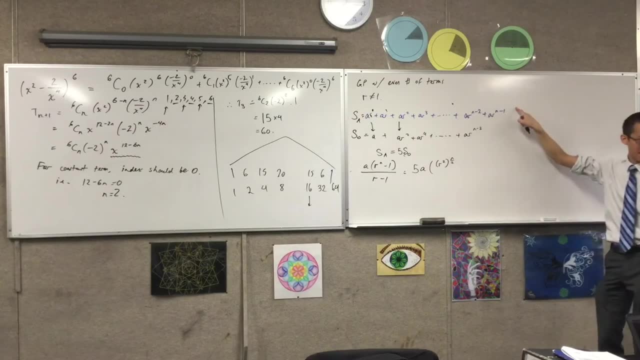 Answer: There are n terms I'm going to forget, Excuse me. There's an odd of zero there, Right? So if I count from here, one, two, three, four, five, six, seven, n minus one, 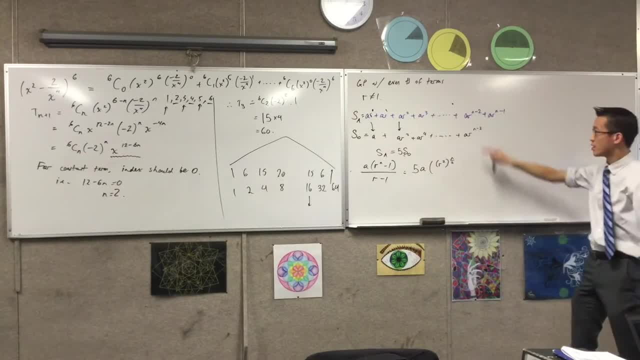 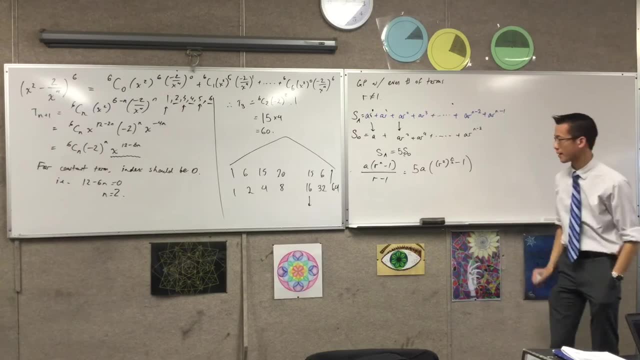 But I forgot that one. So that's the nth term, Right. So there are n terms here, There are n on two terms here. This part is still the same, Okay. And then on the denominator r, squared minus one, Okay. 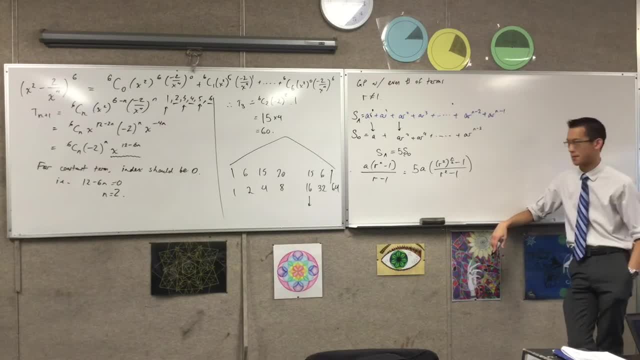 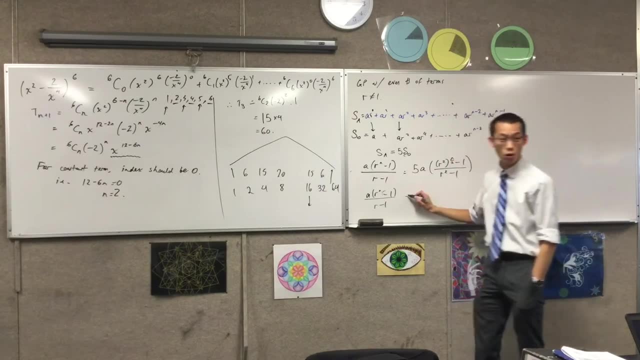 That was all the hard part. The rest of it's just some algebra. Okay, Watch, Watch. as it delightfully unfolds, I'm going to leave this the same, because it will all sort of collapse in a second. On the right-hand side I've got five a. 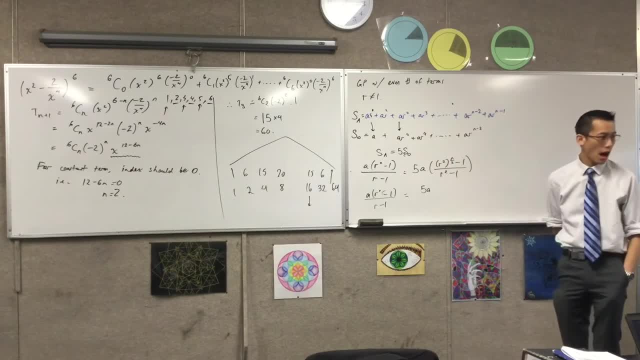 What happens to this guy? That's r to the n minus one, because look at the indices, They just multiply together. So this is r to the n minus one, This denominator. I could leave it like that, but there's a nicer way I can write it: that. 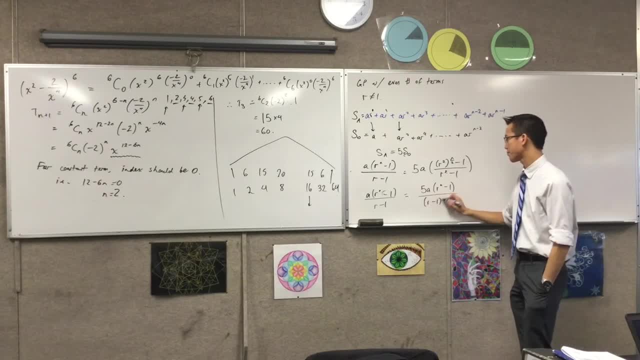 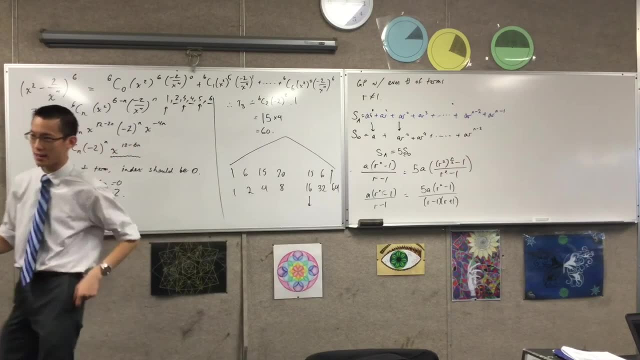 will make the next step easier. I'm going to take difference of squares Right Now. you have a look at this. Okay, Have a look at all those terms on the left-hand side. Every term on the left-hand side is also on the right-hand side. 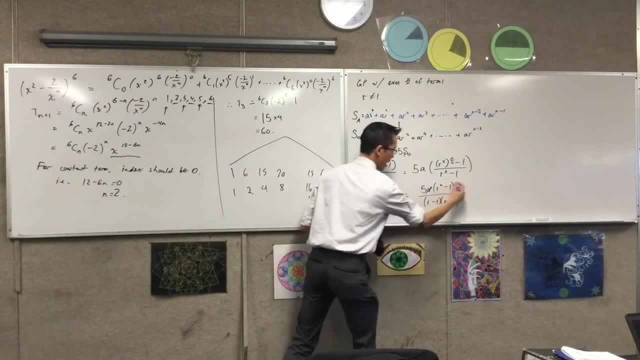 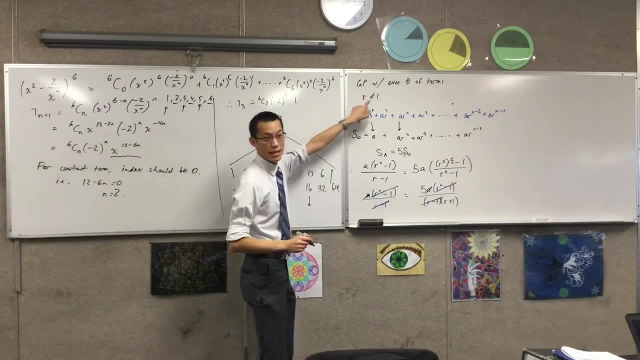 Right, So I can cancel a, I can cancel r to the n minus one And I can cancel r minus one Because, Because, Why can't I cancel it? Because r is not equal to one. They told me that right at the beginning. 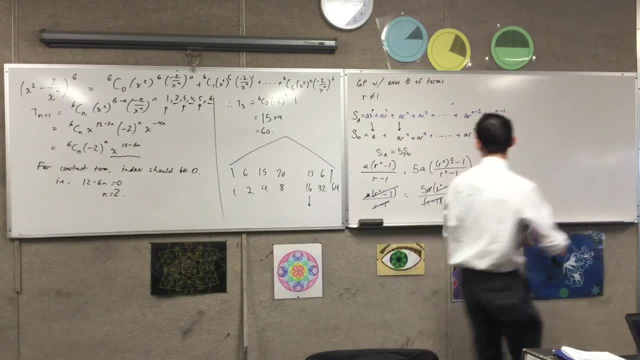 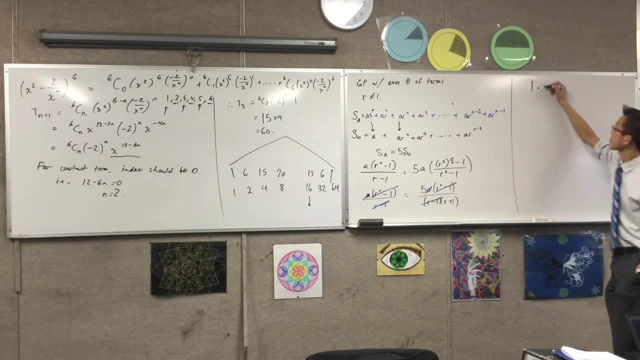 That wasn't just random so that I could do that line. So now, what's left On the left-hand side? I have one On the right-hand side? I have, And what I'm after is r. Yeah, So r plus one is five. 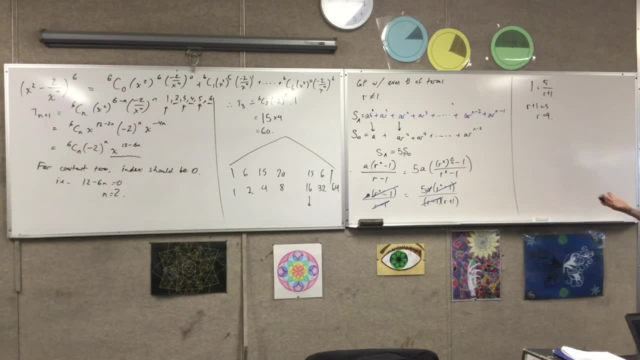 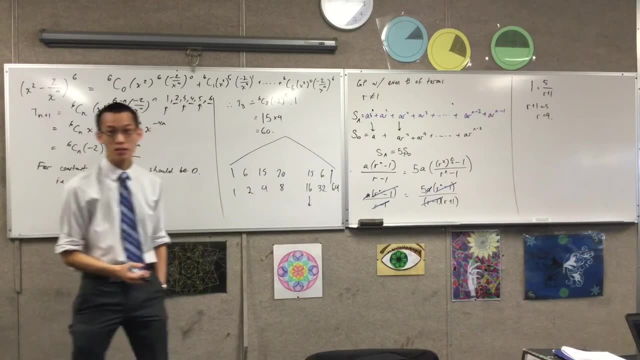 So r is four. Okay, Now I've just gone through all this algebra. It's a weird way to phrase the question, So I'm not all that confident at the moment that I've nailed it. So you know what? I'm just going to test it out. 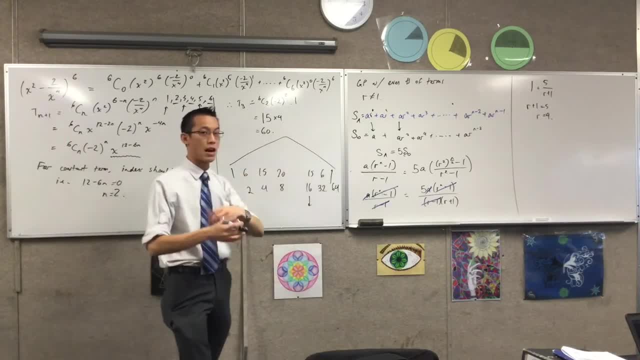 It's not that hard. I don't need to know what the first term is. I don't need to know how many terms there are. That's interesting, So I'm going to give you the independent of those. All you need is the common ratio. 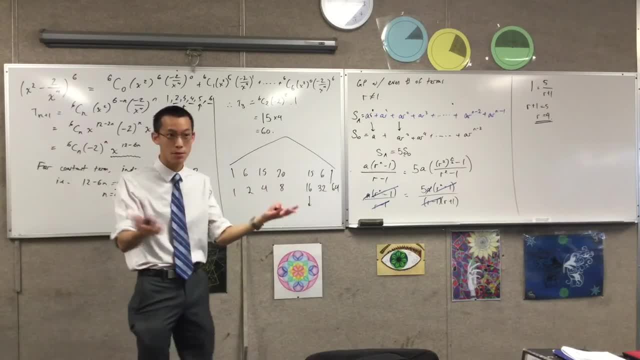 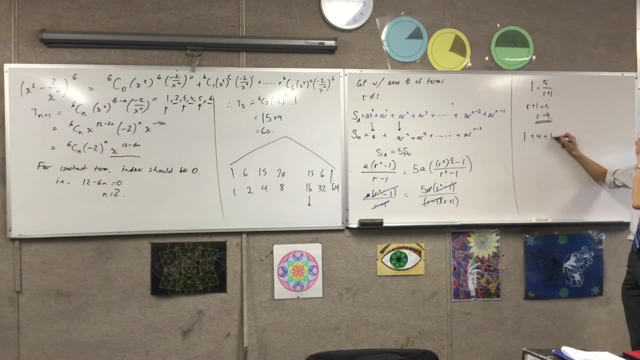 So I'm just going to pick a first term. I'm just going to pick a number of terms just to see if this will work. Right, Nice, easy first term. How about one? Right, If my common ratio is four, then I'm going to get something like that: 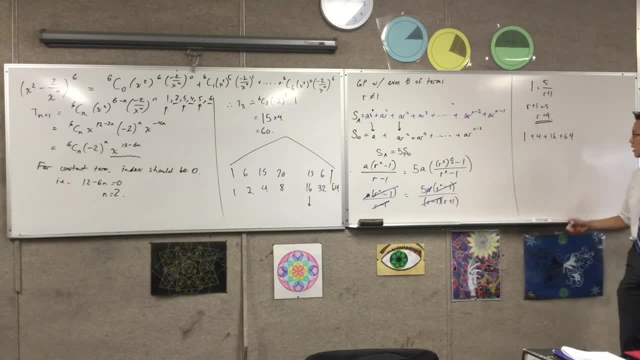 That'll do. That's an even number of terms, Right, Okay. What's this equal to? This is 80.. 85. And that's five. Yep, Okay, Let's pick out the odd terms. now, There they are. 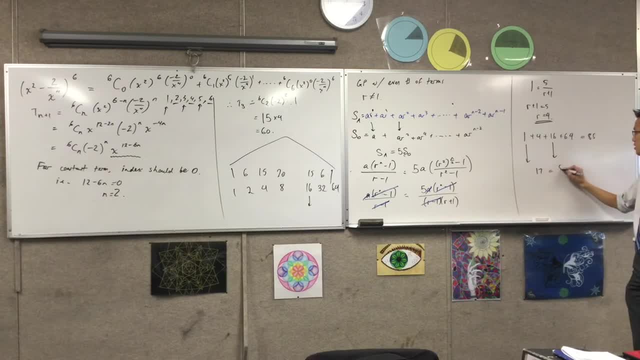 Yep, That's 17,, which is 85 times a fifth. just like I was supposed to get Right. In fact, if you think about it, your intuition should tell you. oh, of course this should work Right, Because what happens when you add the next pair of terms? 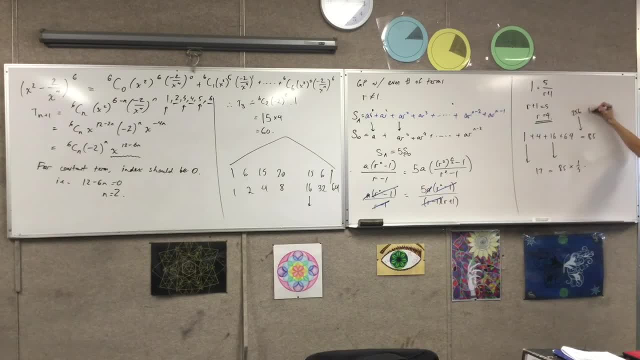 When you add the next pair of terms, the next one will be 256 and 1024.. Do you agree with that? Now, when you think about this series down here, how it's growing, it's going to get that Right. 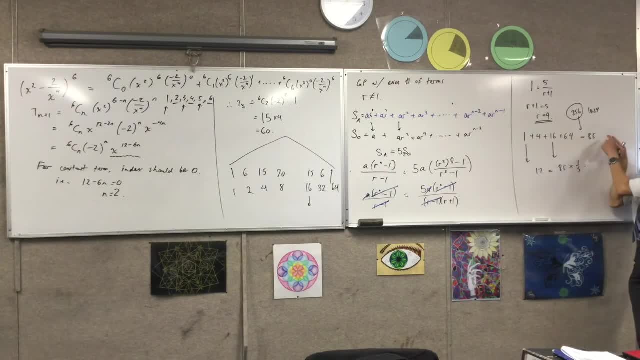 Whatever the next term is, it's going to be four times bigger, Right? So when you think of the big series, you're getting five of them, Right? So every time you add a pair of terms, you're adding this to the little series and you're. 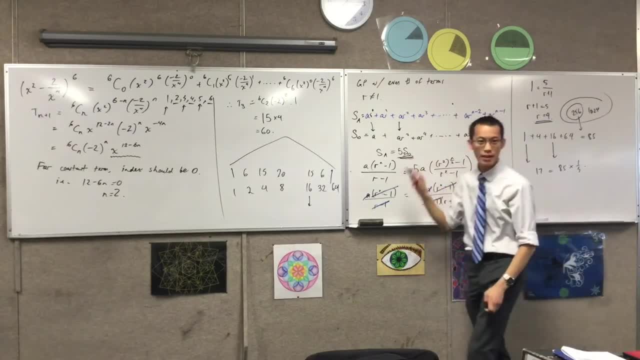 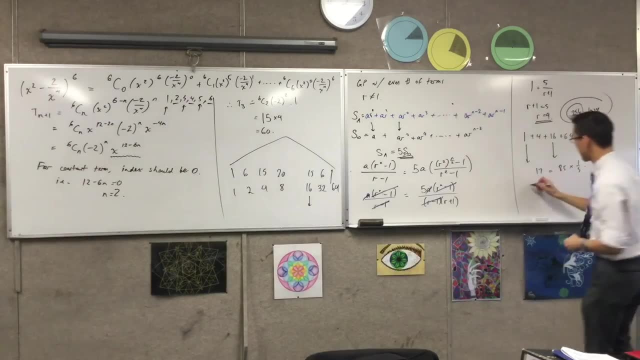 adding five of them to the big series, which is why this is the case. Okay, Do you also have to find the first term? Nope, No, Because I can change it. I can change it. Let's make the series 2 plus 8 plus 32 plus 128. 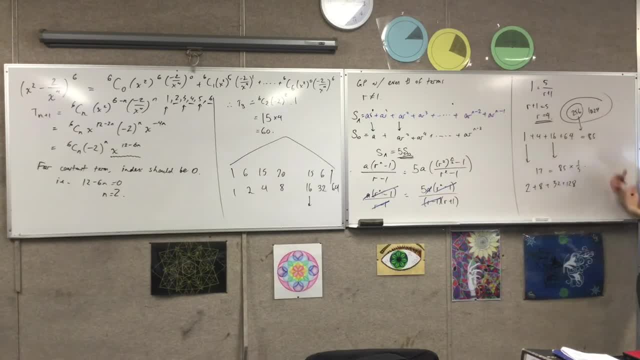 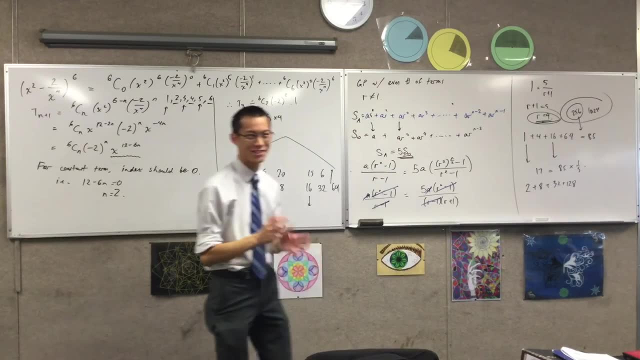 Oh, okay, The same thing, Pat, I just noticed. Right, It will have exactly the same because of this guy. This is the guy that matters. Okay, You can even do it with fractions. I can even do it with fractions if I wanted to, but I don't.